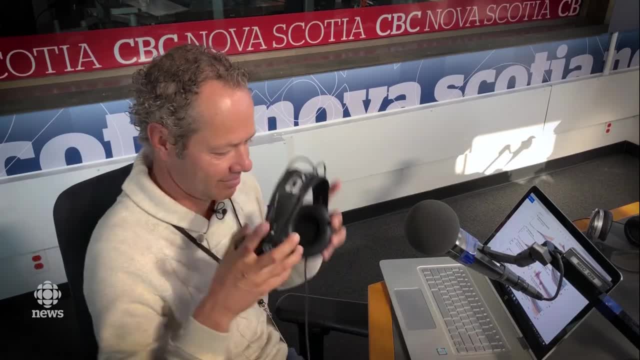 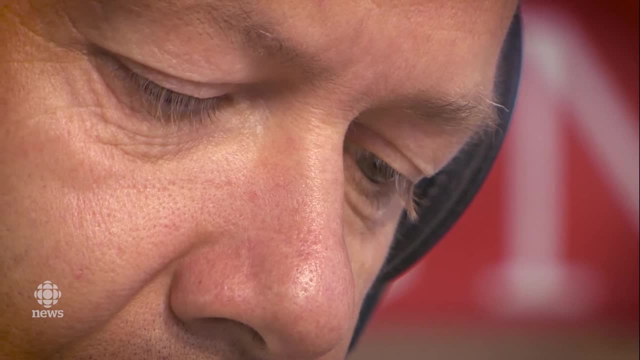 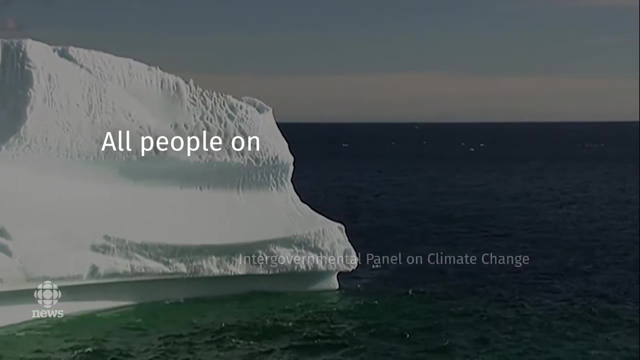 We recorded them and played them back for Boris Varm, an ocean scientist and Dalhousie University professor, And in his straightforward and matter-of-fact way, Boris helped us understand the depths and the tone of the science behind the report. All people on Earth depend directly or indirectly on the ocean and cryosphere. 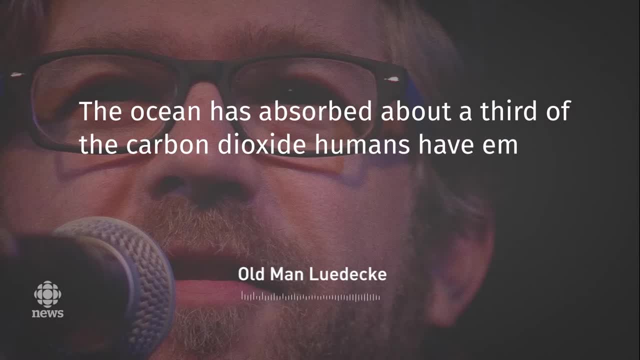 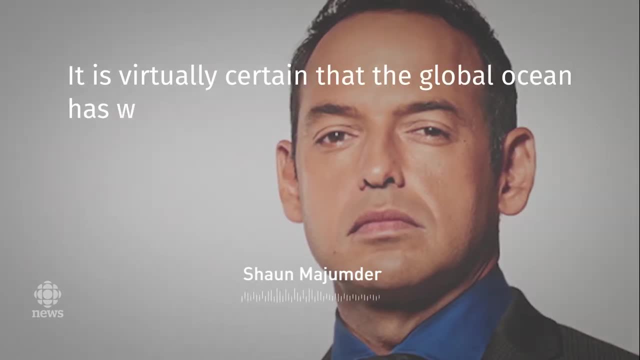 The ocean has absorbed about a third of the carbon dioxide humans have emitted from the burning of fossil fuels since the Industrial Revolution. It is virtually certain that the global ocean has warmed unabated since 1970 and has taken up more than 90% of the excess heat in the climate system. 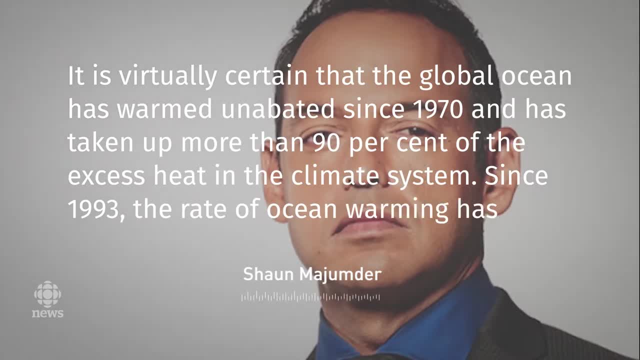 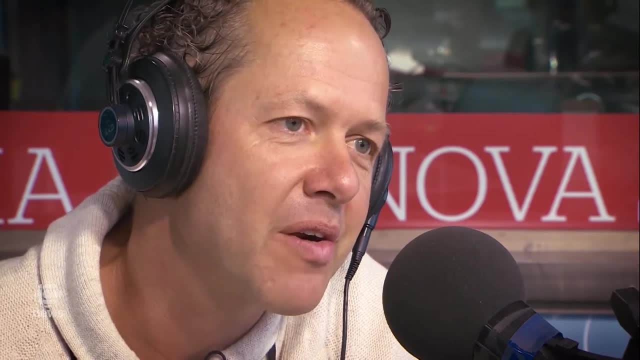 Since 1993, the rate of ocean warming has more than doubled. Well, first I have to respond as a human being, not so much as a scientist, because, you know, this is so much bigger than any of us. The sense of urgency is overwhelming to me. 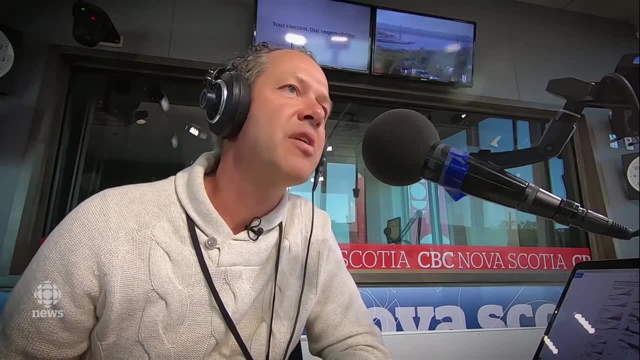 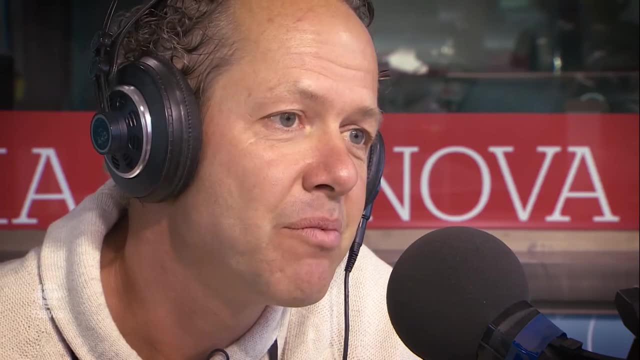 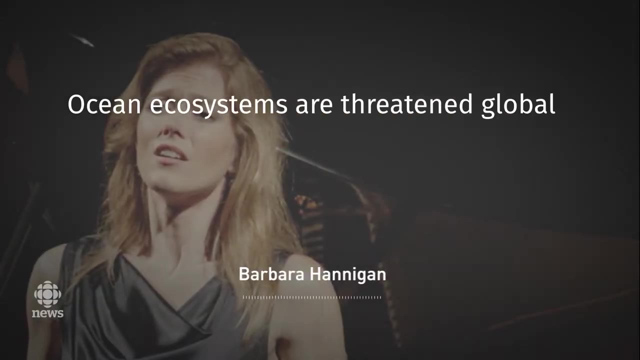 This is bigger than Canada. This is bigger than any political party. This is bigger than any faith group. It's bigger than humanity. It's three quarters of our planet that are part of the oceans or cryosphere. Ocean ecosystems are threatened globally by three major climate change-induced stressors. 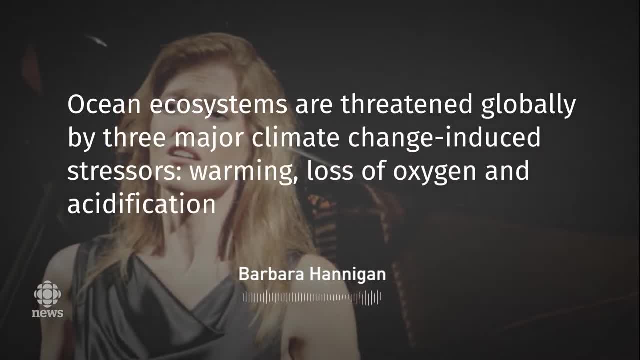 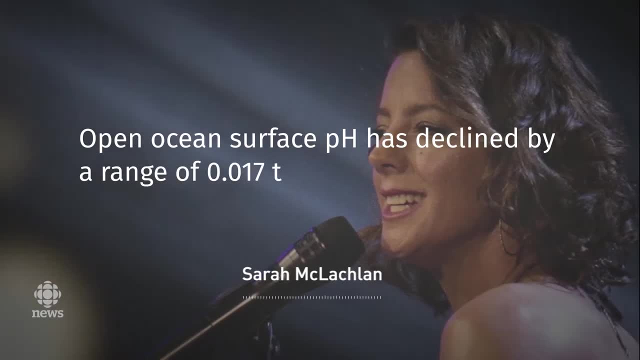 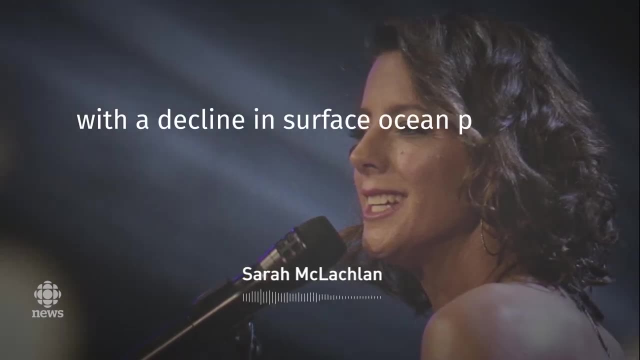 Warming, loss of oxygen and acidification. Open ocean surface pH has declined by a range of 0.017 to 0.027 pH units per decade since the late 1980s, with a decline in surface ocean pH very likely to have already emerged from background natural variability for more than 95%. 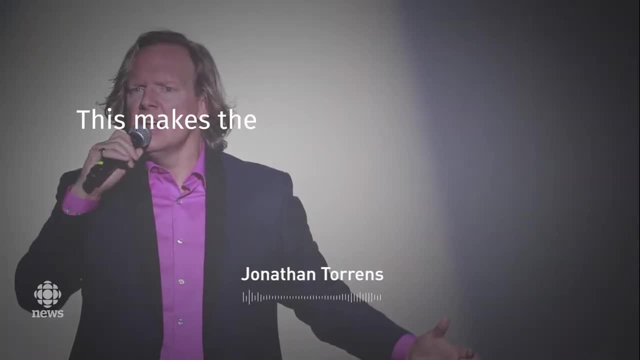 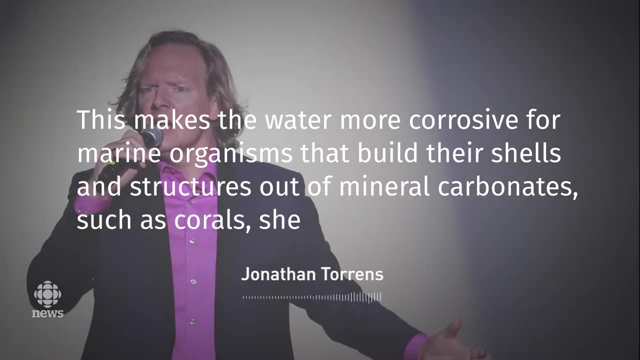 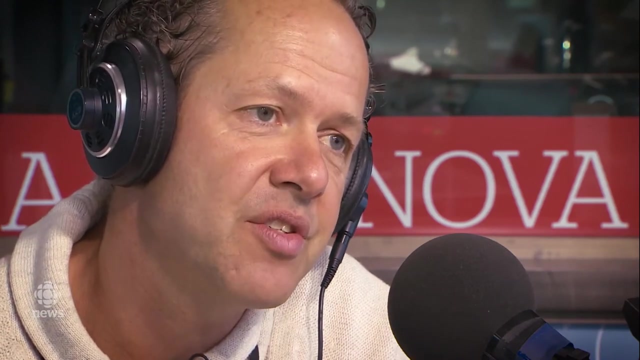 And that's why we're here- The ocean surface area. This makes the water more corrosive for marine organisms that build their shells and structures out of mineral carbonates such as corals, shellfish and plankton. The ocean, on average, is about 26% more acidic now than it was a few decades ago. Now, if our pH in our blood would drop as much as the ocean pH has changed, we would be already quite sick. It's called acidosis. Small changes can be can make you sick. It's called acidosis. Small changes can be can make you sick. 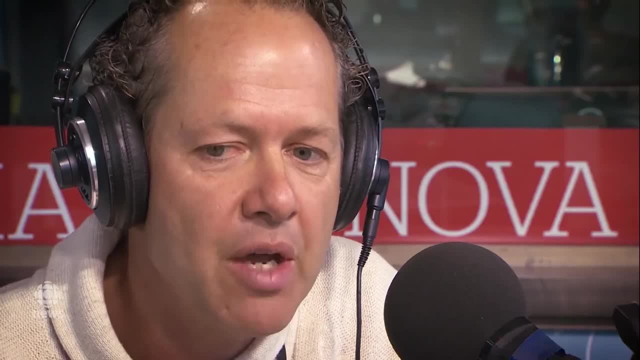 It's called acidosis. Small changes can be can make you sick. The one thing that was hidden in there that I thought was profound was that it said that the oceans have emerged from the natural state. 95% of the ocean emerged.